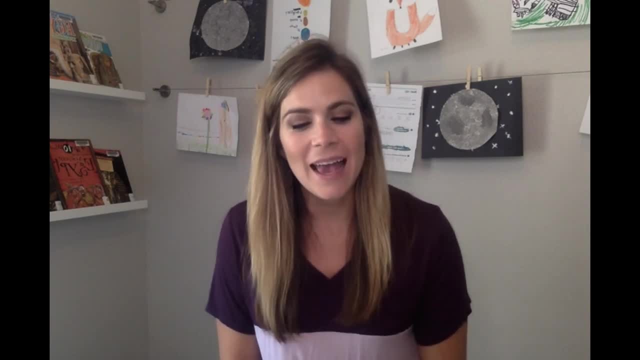 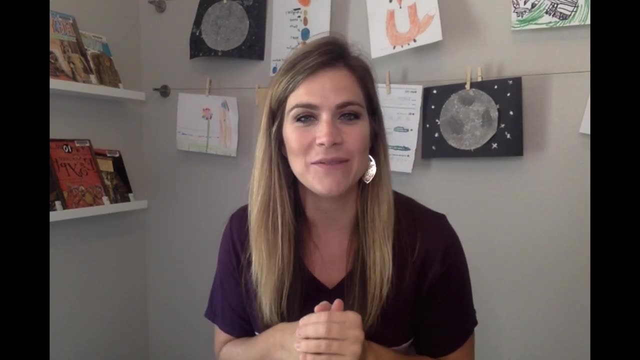 My kids are eight, six, three and almost two And I love talking about curriculum here with you guys. If you're new to this channel, please say hello in the comments. I've had so much fun meeting you guys. It's been a real joy to me to just kind of hear what you guys are doing. 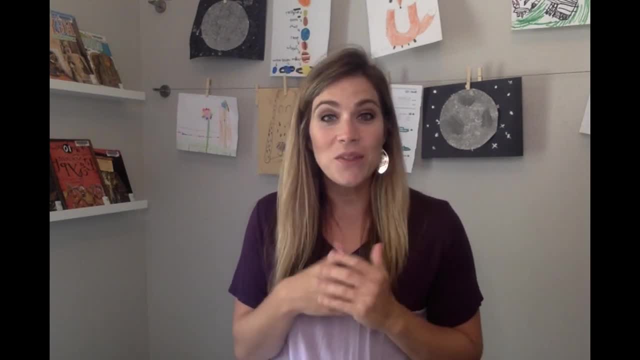 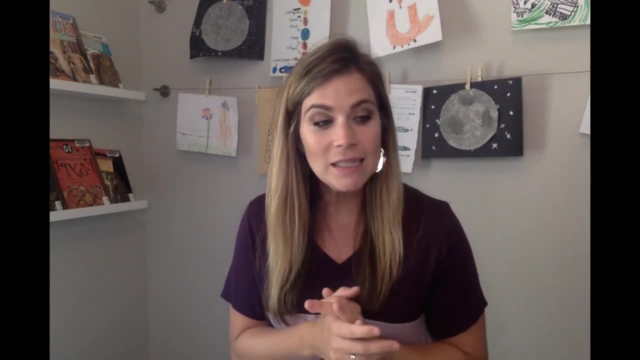 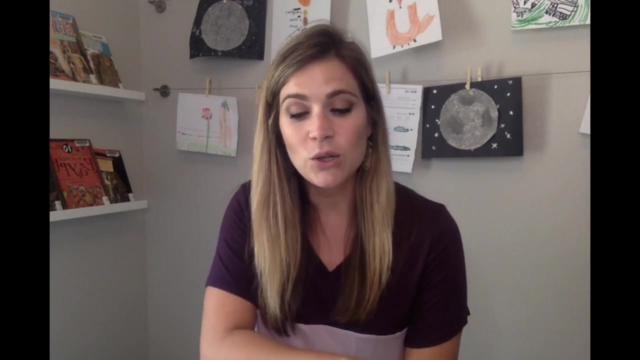 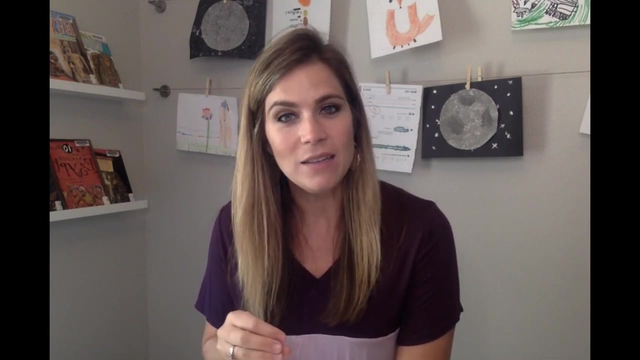 and connecting with a little community here online. This year I changed language arts curriculums for my oldest daughter. She is in the third grade- and we decided to switch from Christian Light Education Language Arts to Learning Language Arts literature. we loved christian light. we were just ready for a little bit of a change and i kind of 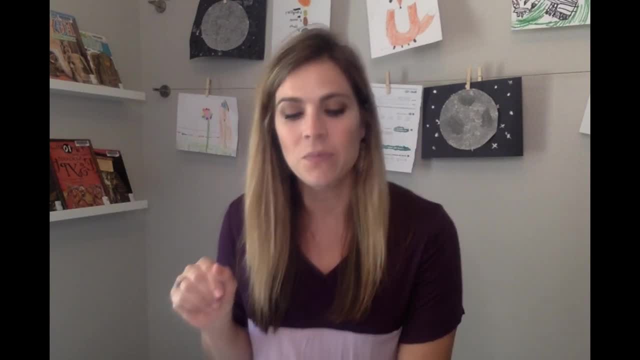 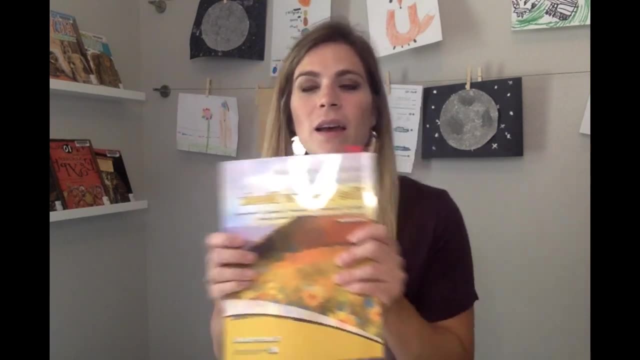 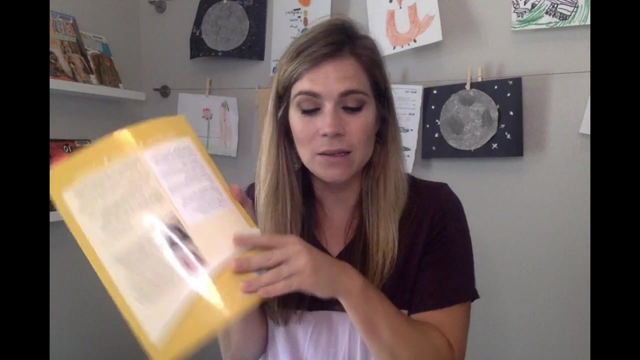 talk about all that in the video so i will link that for you here. well, when i purchased learning language arts through literature, i went ahead and bought the third grade book. so they're organized by color. so the yellow book on the back it'll say like third grade skills. 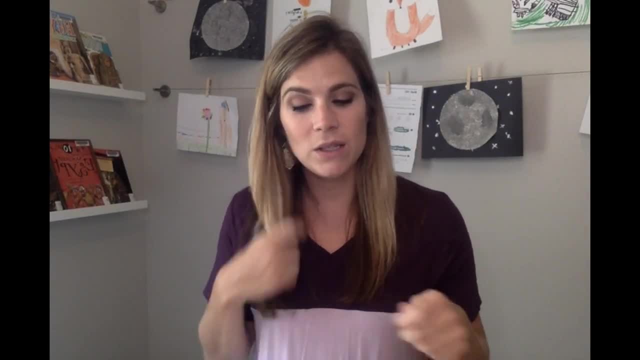 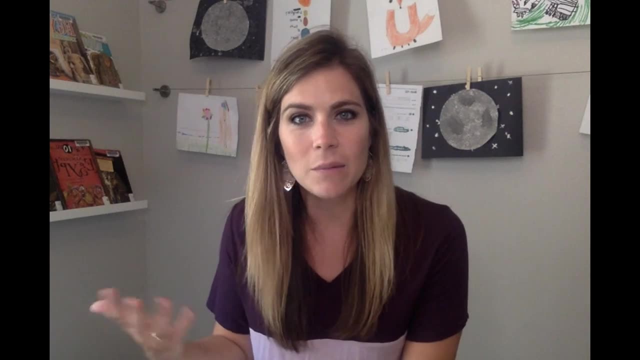 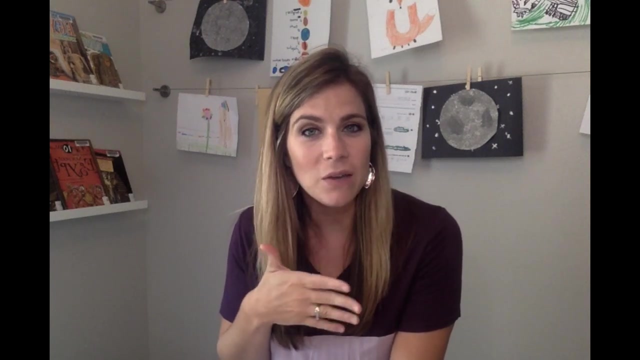 so that's what i got and we got into our year and we started doing the lessons and it was all review, which is pretty normal for any curriculum: the year starts off with review. it wasn't taking us any time to do these lessons and i was actually looking for more time to connect with my daughter. 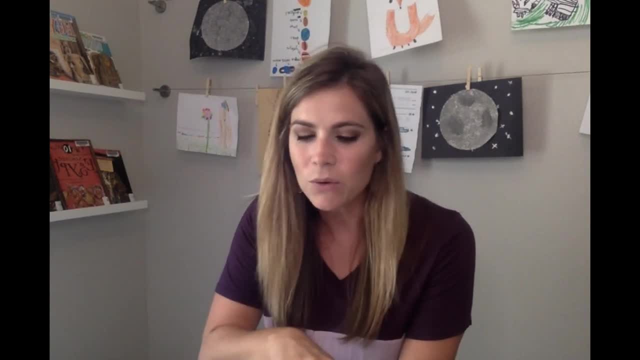 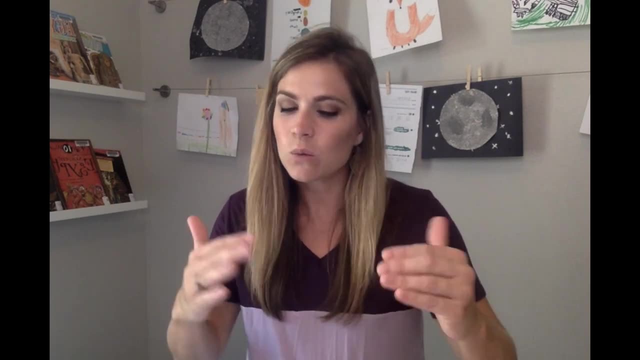 so i thought that was kind of odd, but i mean, we were just breezing through it. so we get to a lesson- it was kind of a first reading comprehension lesson- and you had to read this paragraph and then you have to kind of talk about vocabulary, words and 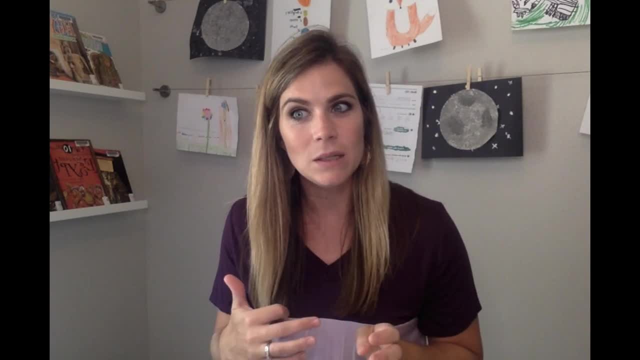 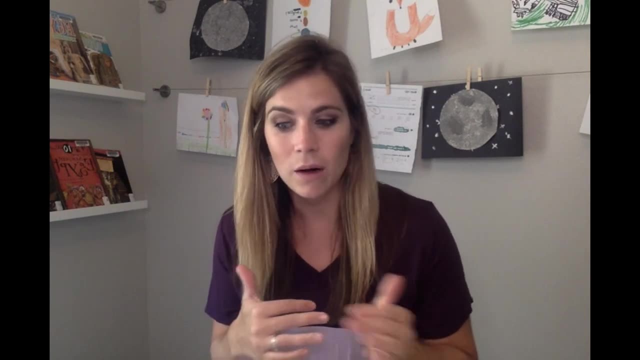 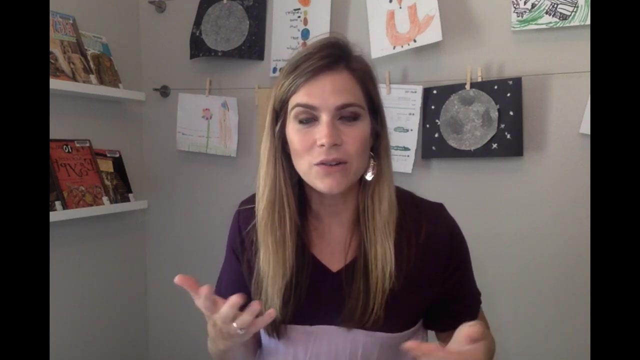 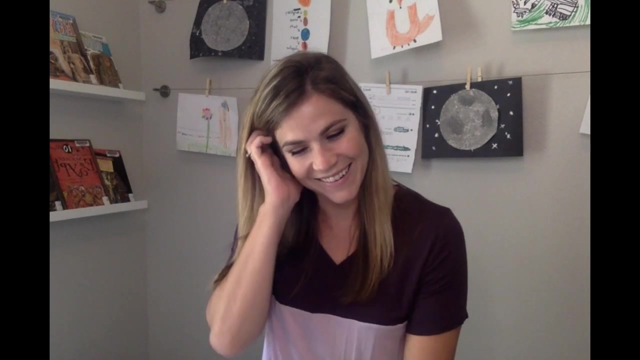 answer questions. well, the vocabulary seemed way too easy, to the point. I mean it did say pick words that you want to work on, but I mean they were all really simple words and so I just thought I'd ask her a few so we could do something. and she looked at me like are you serious? and I'm just like trying to stay. 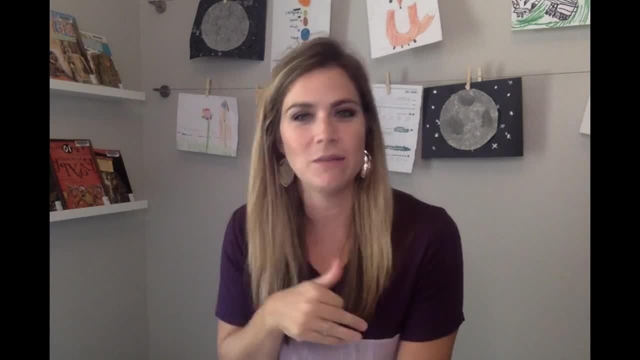 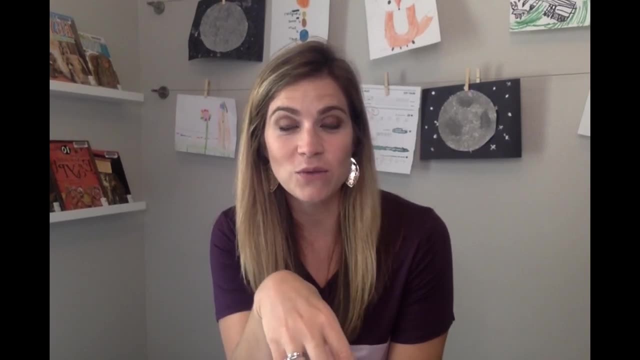 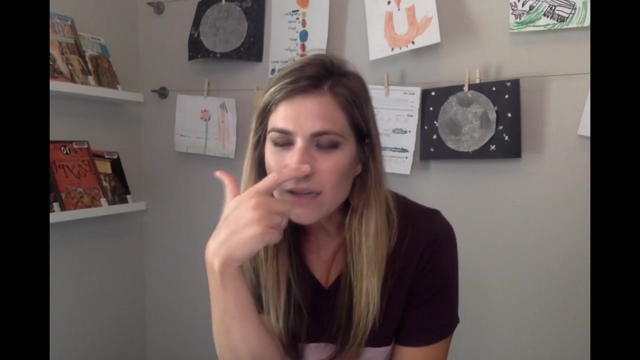 positive and then I'm like: okay, it's just vocabulary, maybe she just has good vocabulary. so then we go and we take the, we answer the questions for the reading comprehension and she answered them just fine. so then I start thinking what is going on here? because she was upset, she was frustrated and I could see it in her. 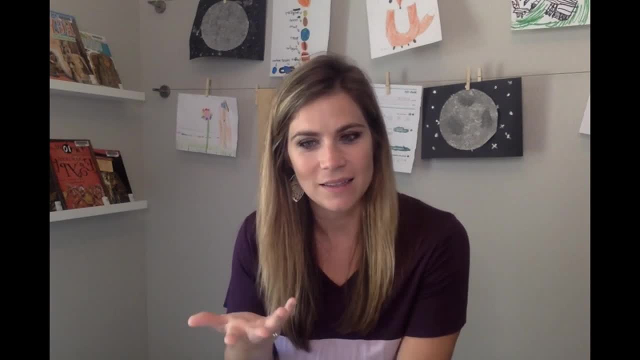 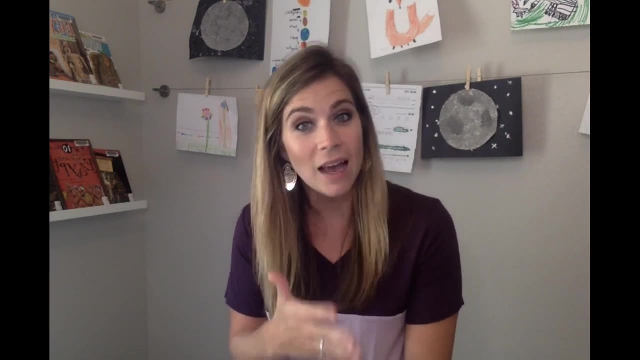 head and I started thinking is: is she thinking like? this is not any fun? not that language arts always has to be fun, but you know you want to be challenged and she's a kid that likes that. she likes the challenge. so I start flipping through the book and I think to myself: maybe the vocabulary gets harder in the 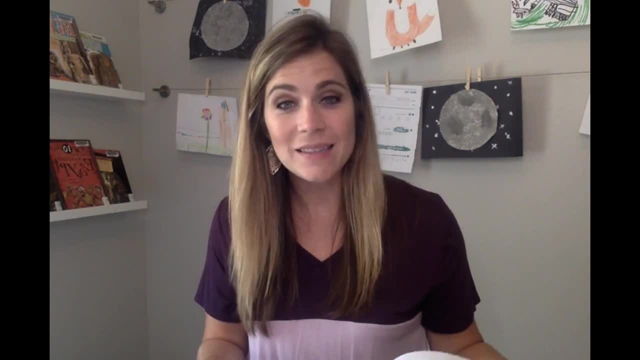 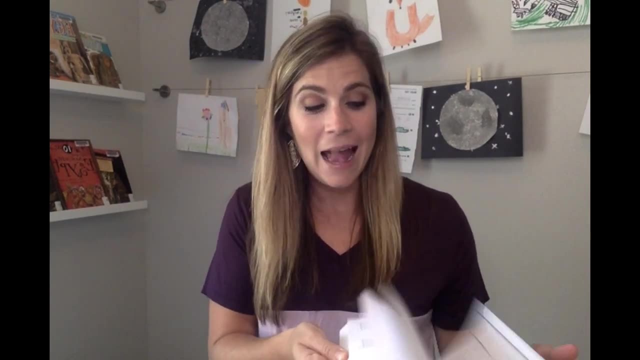 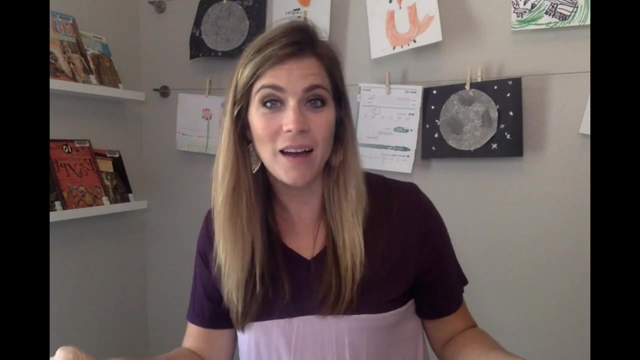 back. it really didn't, and I thought: what are these lessons consisting of? and so I start, you know, looking at the lessons, what she's going to be learning and everything in this book. we already covered for Christian light language arts 2, so I thought, oh my. 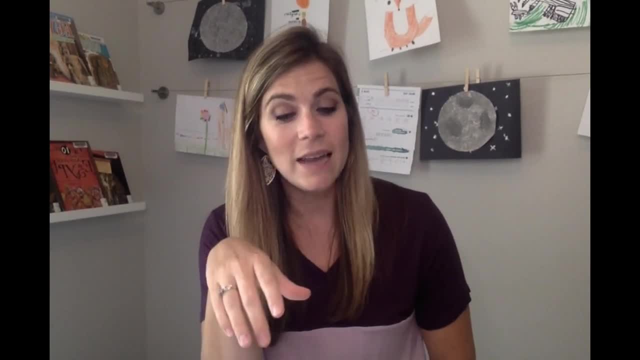 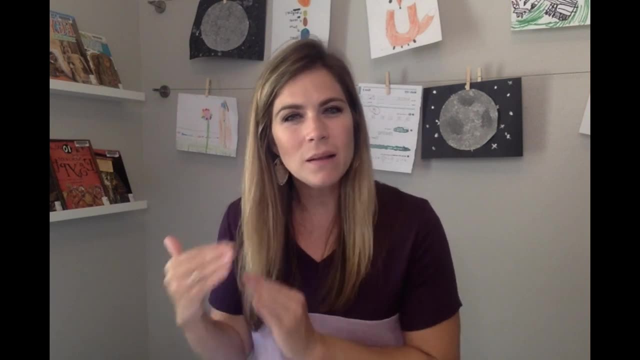 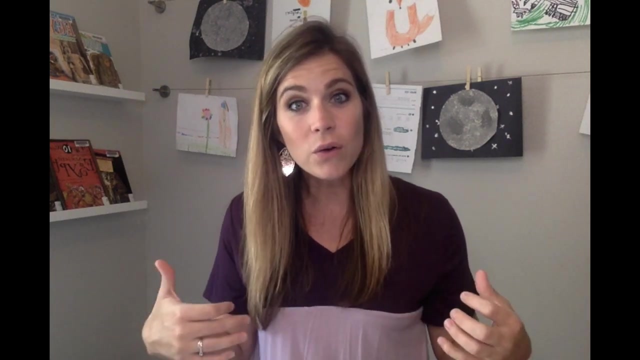 goodness, this was the wrong book. now I have switched curriculum once before, but my child was in first grade and it was in the middle of the year, so it wasn't really like a big deal. this was the first time that we now she's in third grade, so we've had a few years behind us. 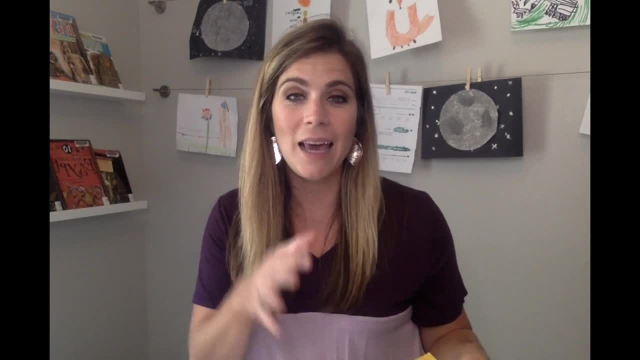 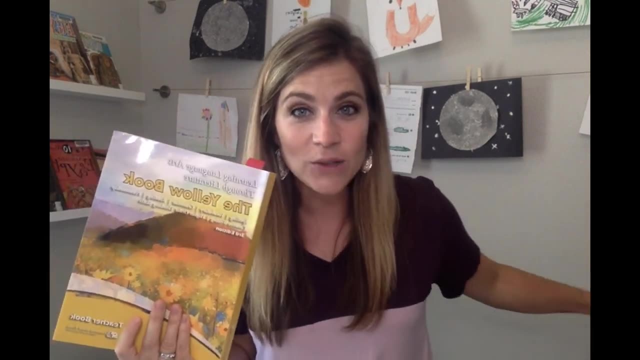 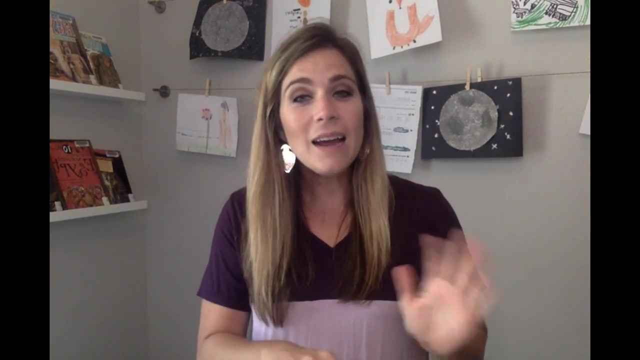 I didn't realize how important it was to take the assessment, because when you're comparing learning language arts 2, literature in Christian light education, they are very different. I kind of had a little bit of a panic, thinking what are we going to do? and then I started. 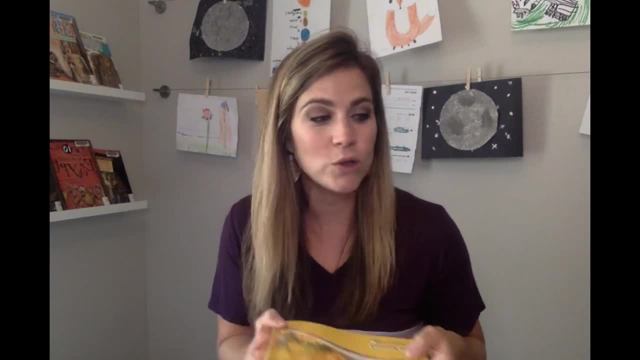 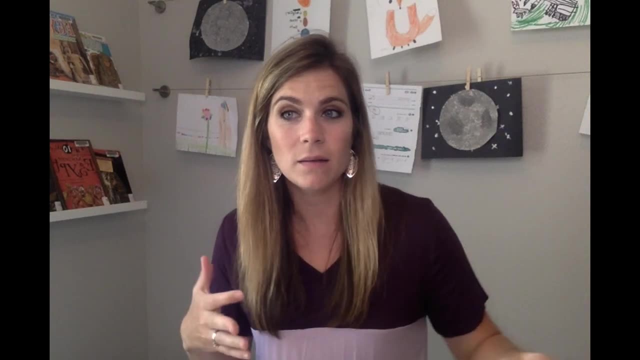 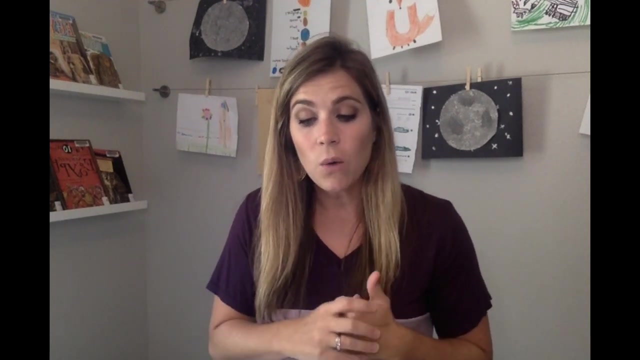 second-guessing myself: should I have really switched or should I just tough with language arts? so I went online and I looked at the to figure out which one would she really need, and it turned out it would just be the next color. so the next color was orange. so I thought to myself: okay, I'm going to go ahead and order the. 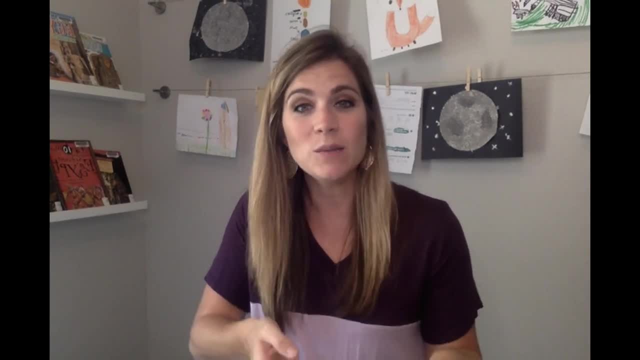 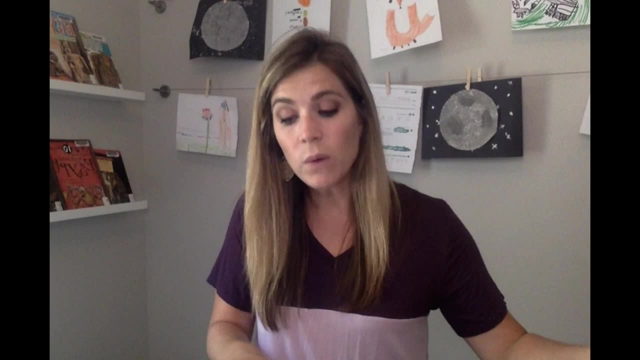 orange. but I'm only going to order the teacher's book. I mean, at this point I've already spent almost 70 bucks for two books, so I only ordered the teacher's book. and while we waited for the teacher's book, we went through and took the assessments in the yellow book, just to kind of. 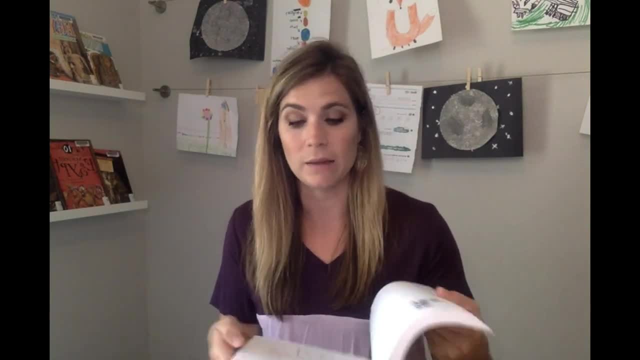 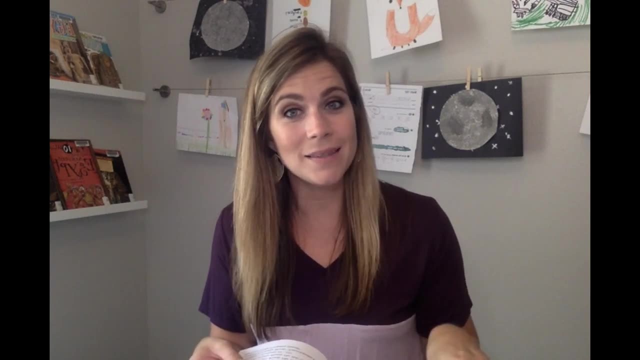 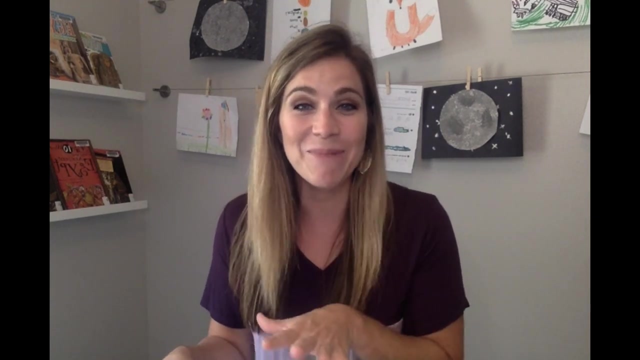 give myself peace of mind that she really was knowledgeable about these topics. so there are eight assessments in here. we completed five assessments in about 20 minutes and then we did the next three the next day, and so it was like: okay, I feel really good that this was probably. 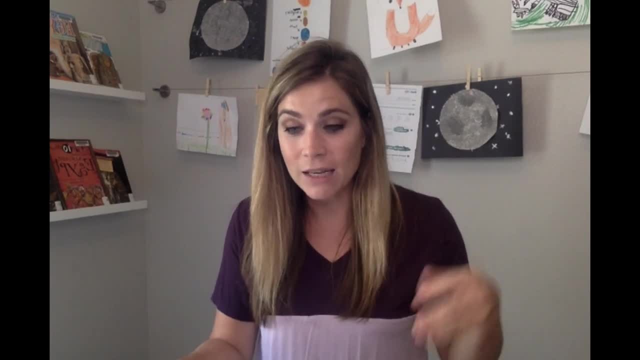 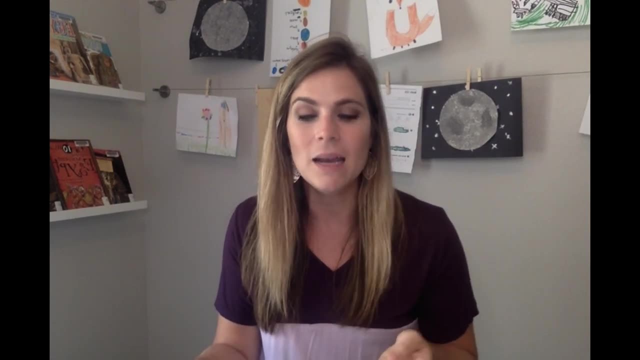 too easy. it's just proof that when you change curriculums, a lot of things can be different. and- and now saying that out loud, I feel it's like an obvious statement, but I had just never experienced that before. so I'm going to give myself peace of mind that she really was knowledgeable. 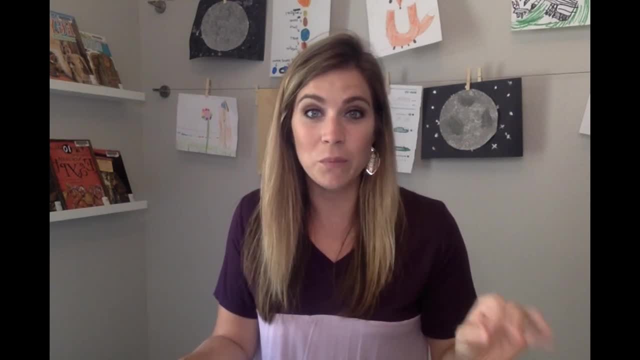 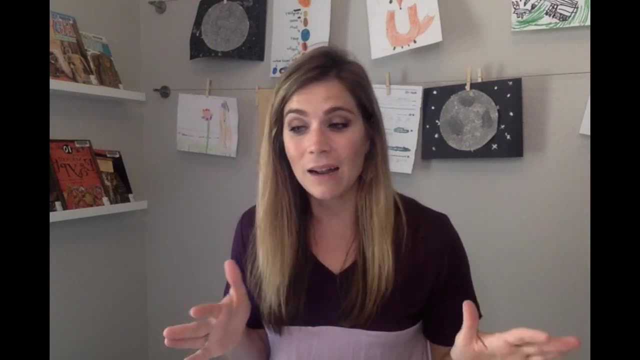 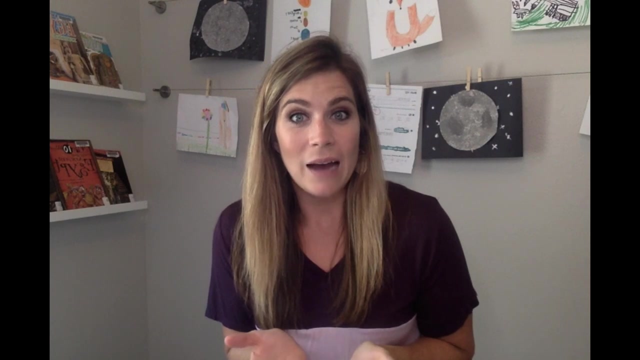 it was definitely a learning moment for me, so I had a couple of thoughts about all this. I'm not interested in trying to get my daughter like way ahead- that's not a goal of mine at all- but I am interested in challenging her and I have the flexibility to do that as a homeschool mom. so 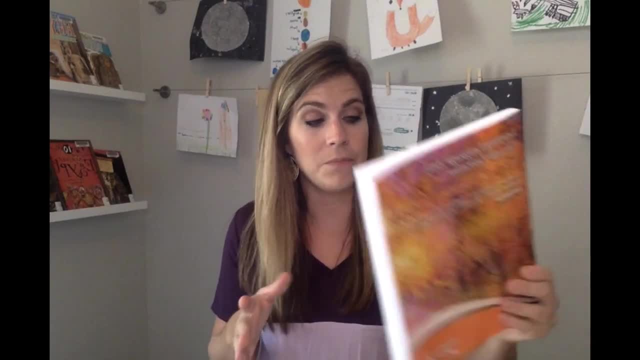 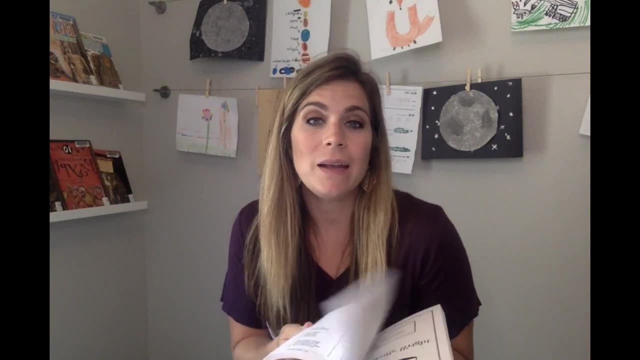 I decided to just go with the next one, which is technically fourth grade skills, but we're just going to go with it and work our way through it, and I'm going to give myself peace of mind that we're going to get it at a pace that seems comfortable. the other thought that I had, though, 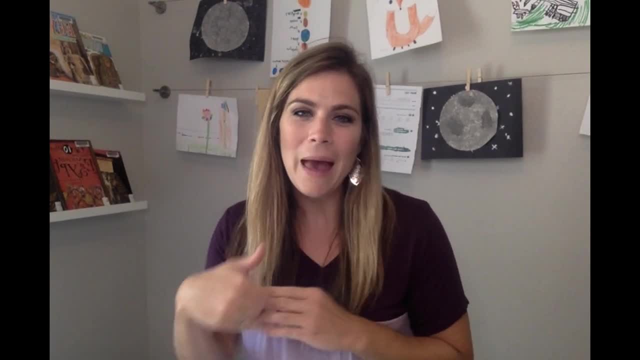 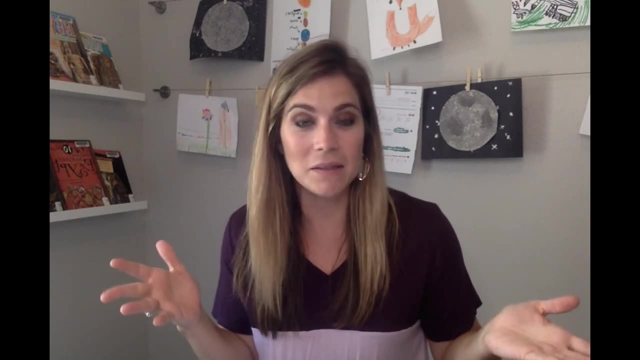 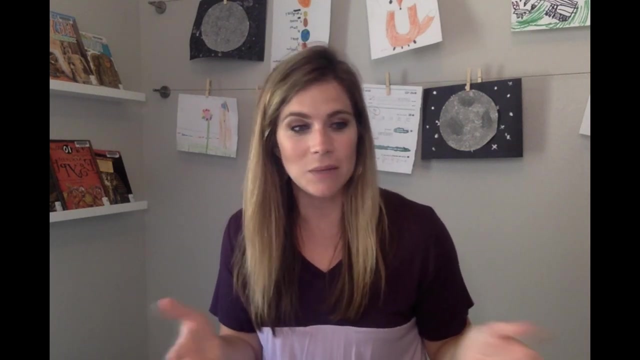 is now. am I setting her back? because it seems like Christian light was pretty advanced. I guess is the term that you would use and that never really occurred to me before, but now, comparing it to this, it kind of seems like it was. I guess I could admit to a fear that I had, was and now am I. 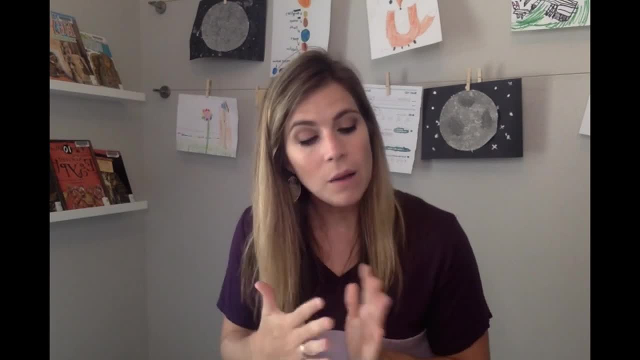 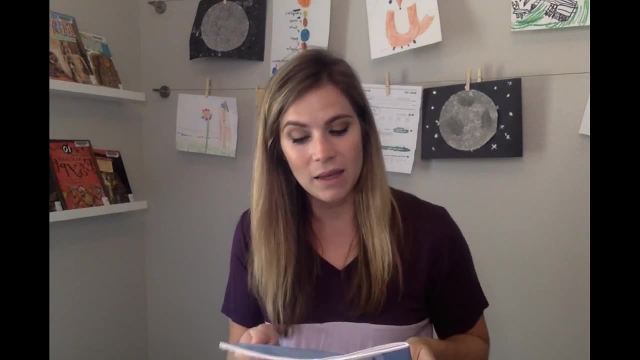 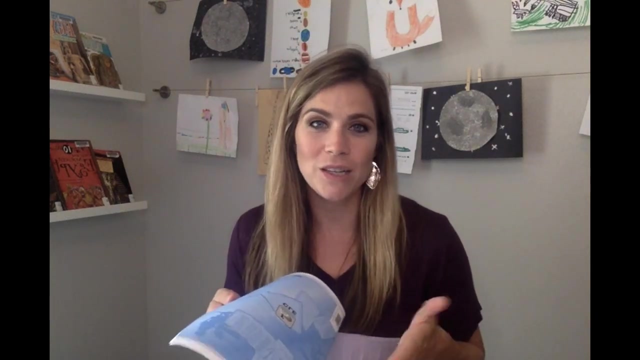 not challenging her enough. I kind of thought about what I wanted to do for that. now here's my solution. Christian light has something in their program called extra practice sheets, so it's literally just worksheets, which I'm not a super fan of, but it's going to cover the skills that would have covered in their third. 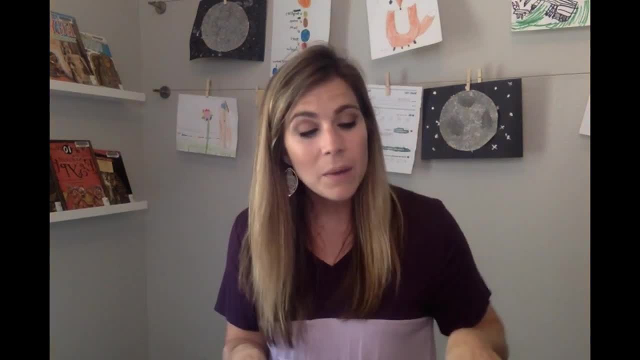 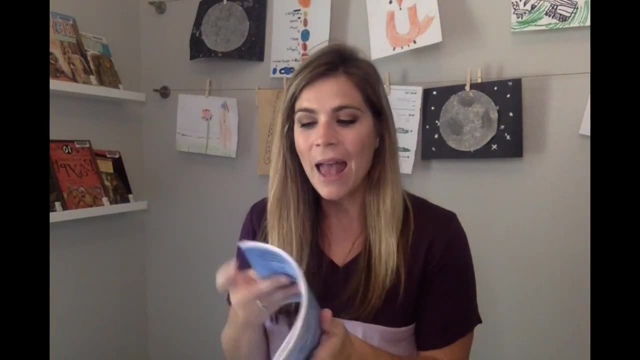 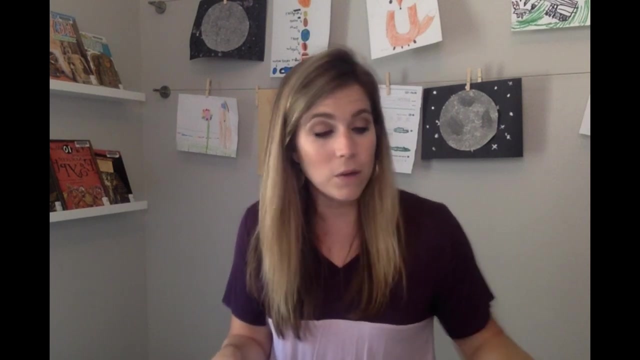 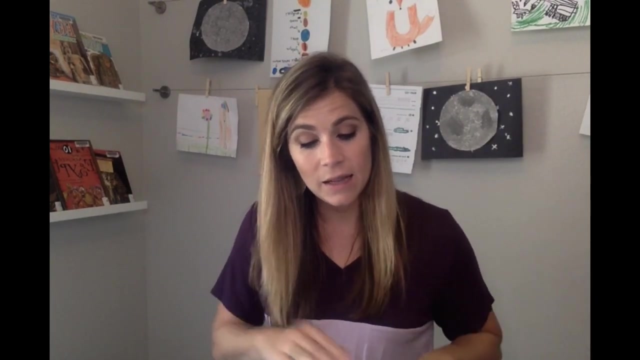 grade program and it cost me four dollars. when we come across different skills in here, I can reinforce it with this. this is actually really nice. it's not super big. there's not a lot in here, but you know, for example, today we are talking about capitalization in our orange book and in this worksheet there's a little. 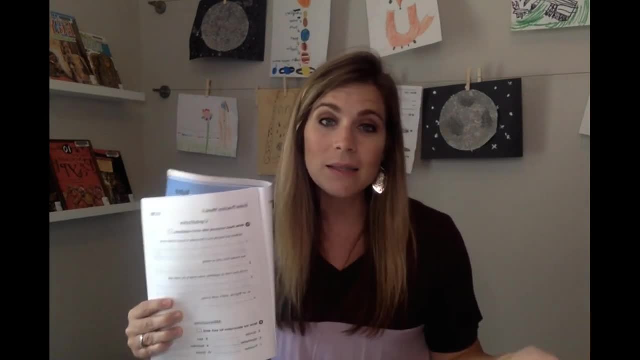 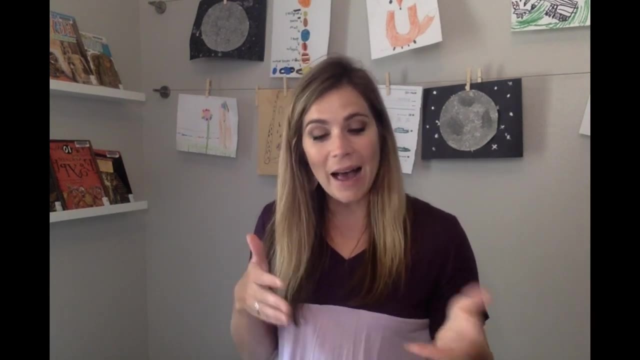 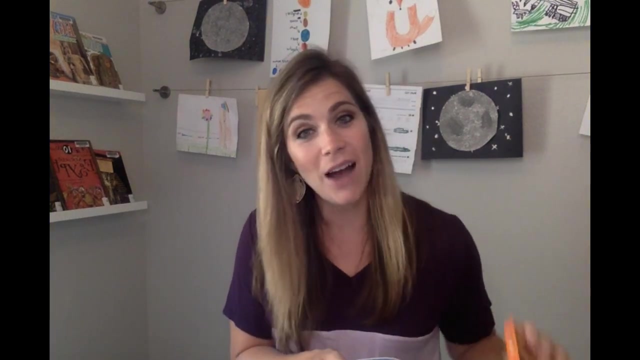 section on capitalization. so if I wanted to practice some extra, I could. there are times when this book will say things like practice more examples, and so I, if I wanted to, I could just grab this book instead. now there are things in this Christian life book that are not in this book. 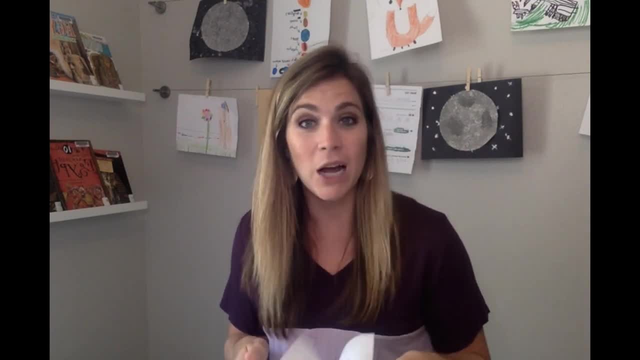 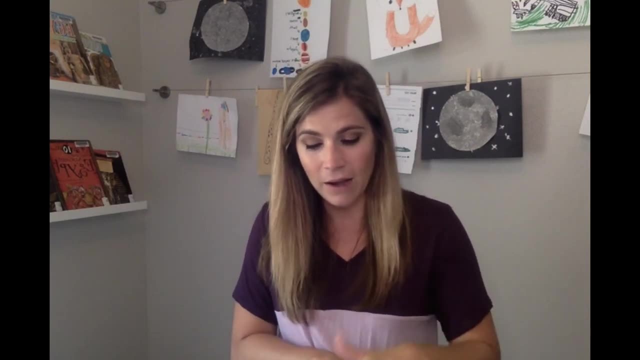 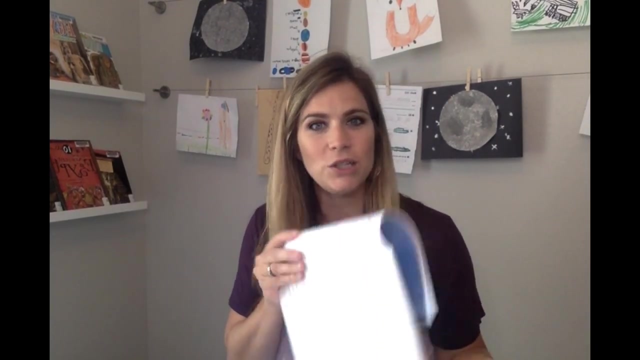 specifically I'm talking about diagramming sentences. I, when I was a kid, I love diagramming sentences. I thought it was super fun, and my daughter and I are very similar in some ways and I think she really might like it too. so I thought at some point, if we wanted to, we could kind of touch 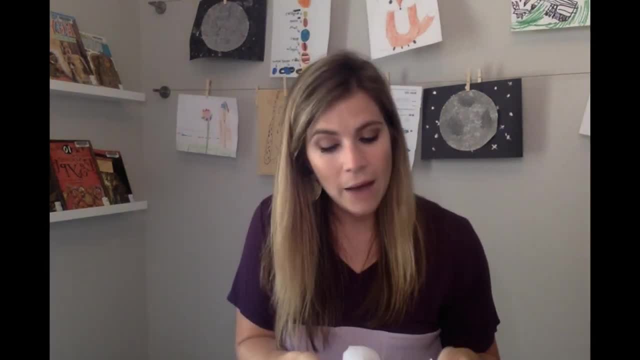 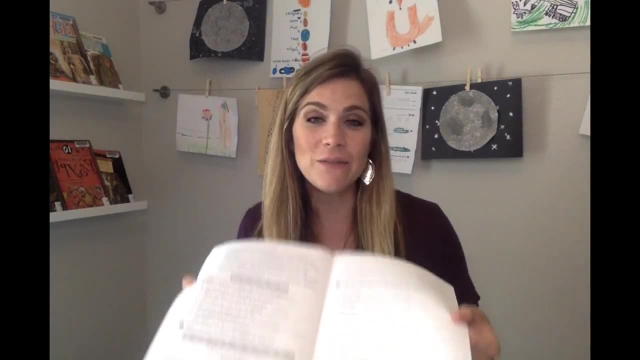 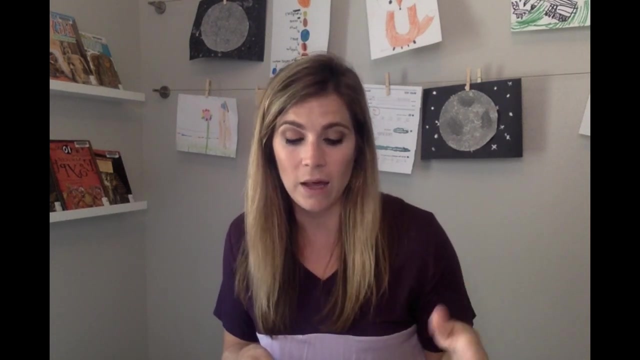 on diagramming a little bit in here. so now I'm gonna talk about the diagramming and I'm gonna get- I don't have set in stone plans for these extra practice worksheets. Honestly, it was $4.. They're here if I need it. And then it really allowed me to see different skills that she would have practiced if we would have stuck with the language arts level three. 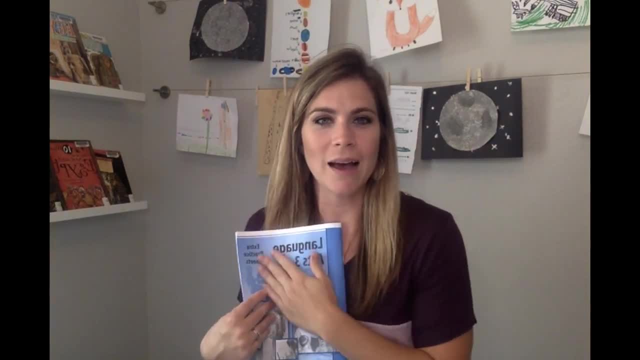 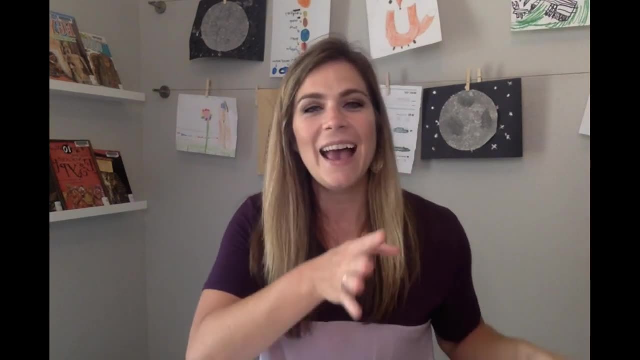 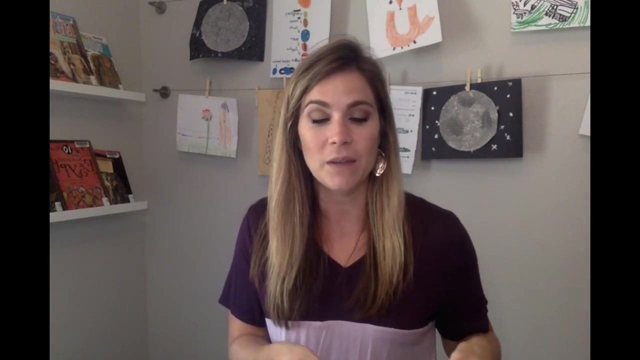 So this was kind of just more of like my comfort. I was feeling kind of guilty for switching, because we really did love this, but I thought change was necessary And so it was kind of my way of: okay, this will be fine, We'll kind of just supplement a little bit with their extra practice. 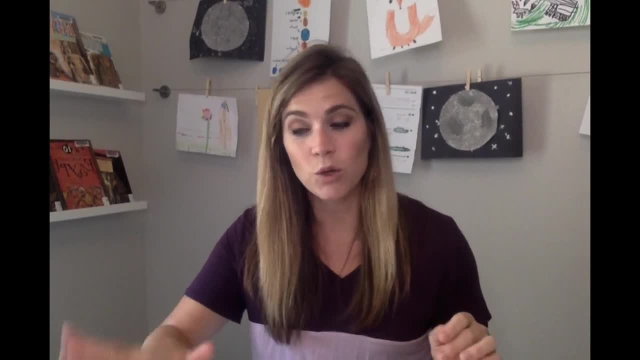 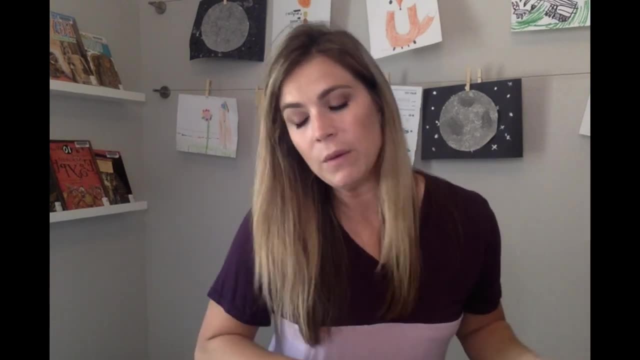 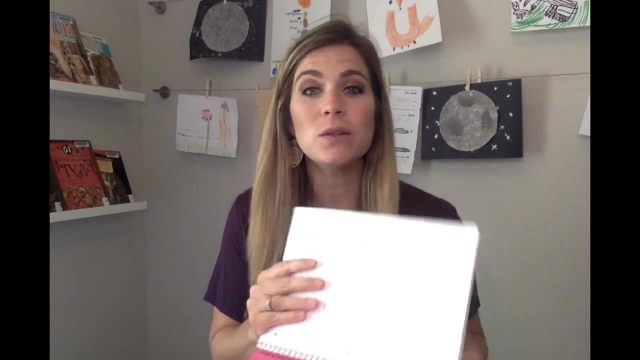 To save money, since I spent money on the teacher workbook and the student workbook. we are just doing the teacher workbook. I've seen somewhere- I can't remember where if it was on YouTube or there was a website- You can do this curriculum with a notebook. We have started doing that and it's been great. She writes her passages in a notebook. If there's spelling words we want to practice, we put them in there. 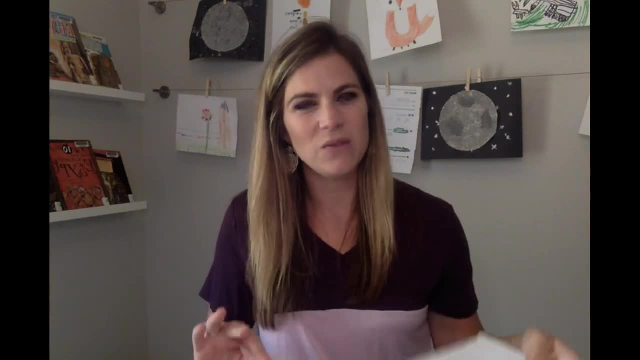 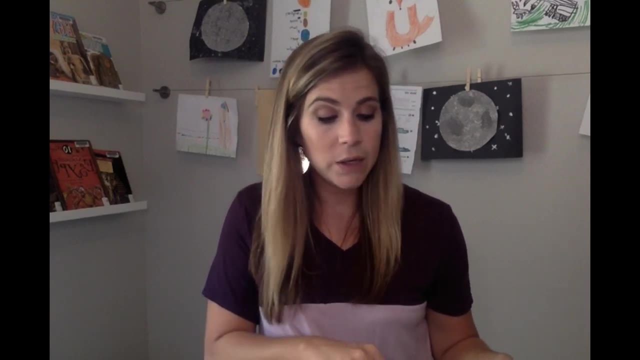 If there's new vocabulary things that I don't think she's very familiar with, I'll have her write it in there and there's a glossary in the back so she can copy vocabulary words. Sometimes we'll put examples. Yesterday we talked about adjectives and we wrote a couple examples. 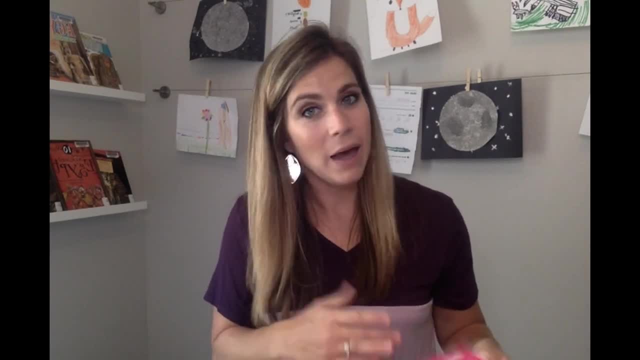 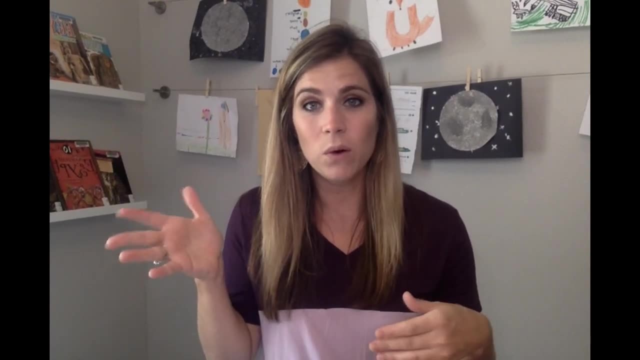 So it's just kind of When I feel like it would be helpful for her to write it down, we put it in the notebook. Otherwise, we just kind of answer questions verbally or we have a whiteboard and we put the answers on the whiteboard and she likes to get up and do that. 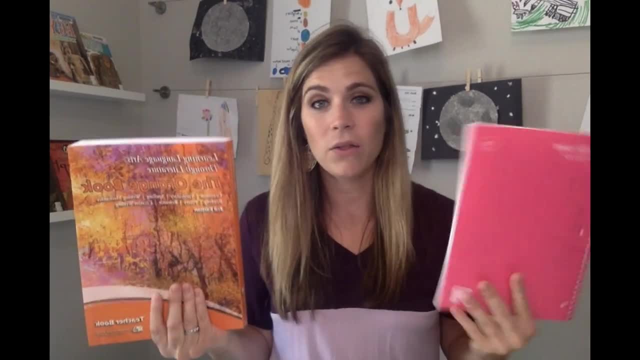 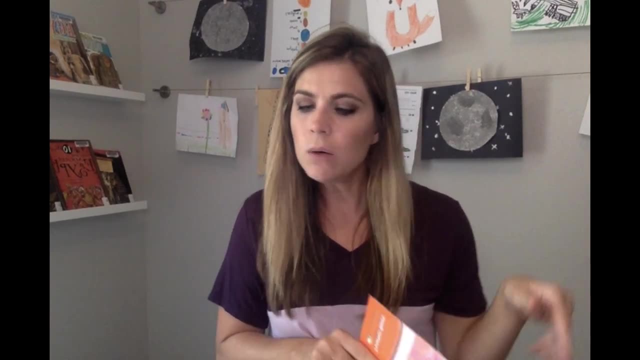 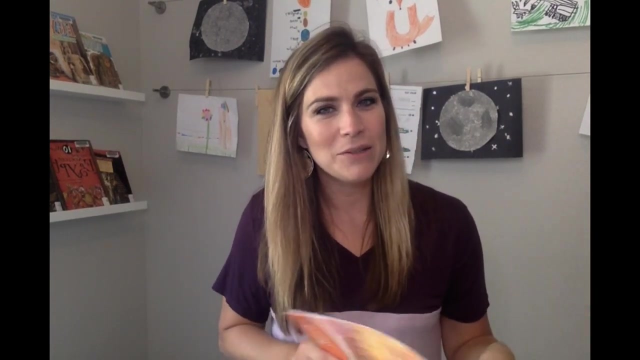 So we're going to do this whole thing with just the notebook, no student book. So really the only thing we're missing out on is the student workbook has enrichment activities like extra things you could do, And honestly I would probably let her skip those anyway, so I'm not too sad about that.